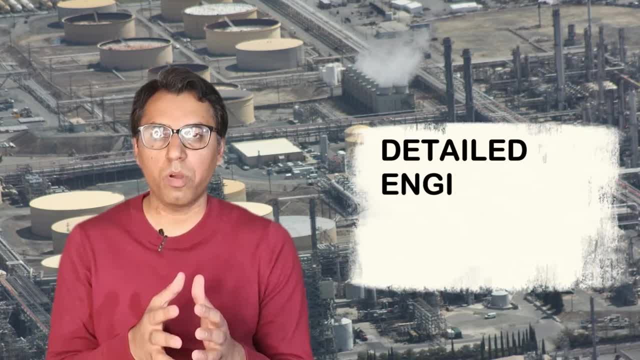 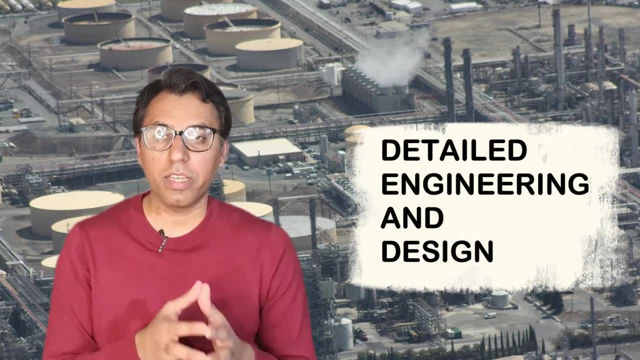 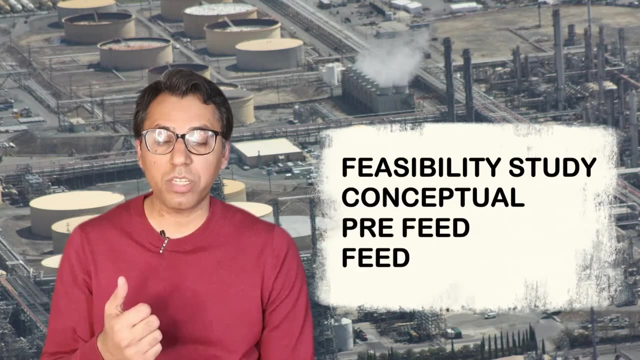 Hi everyone. In this video I will talk about detailed engineering and design. I will talk about its definition, its inputs and expected outcomes or deliverables. Detailed engineering and design come after completing feasibility study, conceptual development, pre-feed and feed of any particular project. 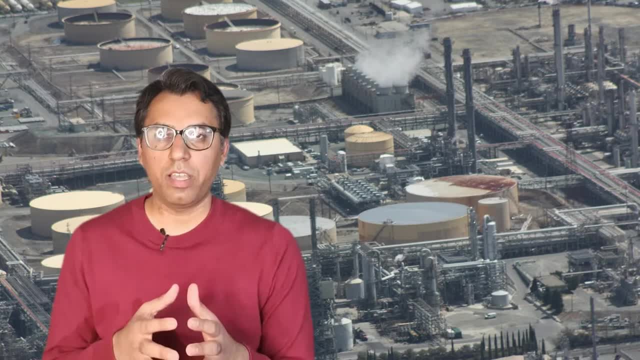 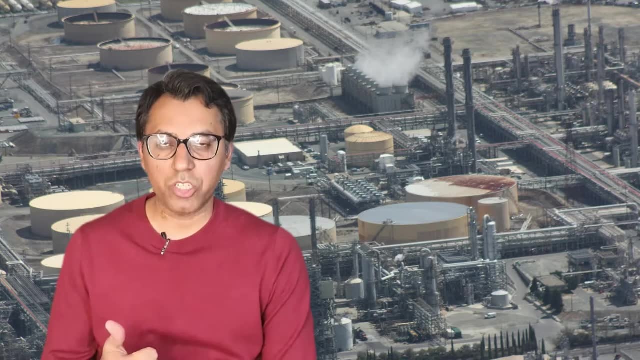 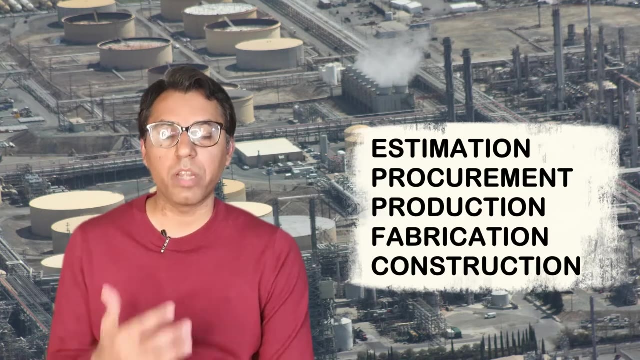 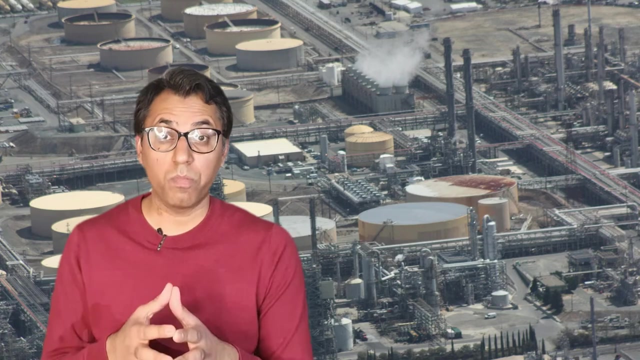 In a nutshell, detailed engineering and design involve all the calculations and drafting to provide exact drawings in detail for the estimation, procurement, production, fabrication and construction of any particular project. Normally, an EPCM contractor company is engaged to perform detailed engineering and design. 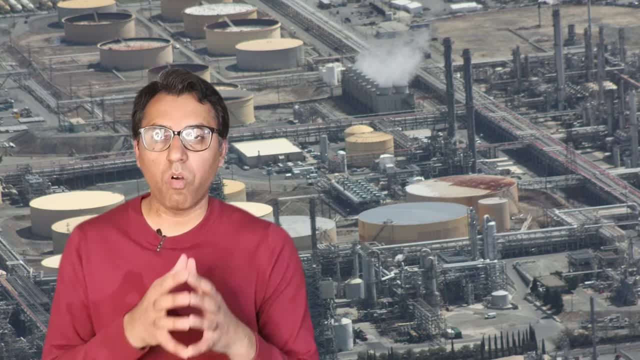 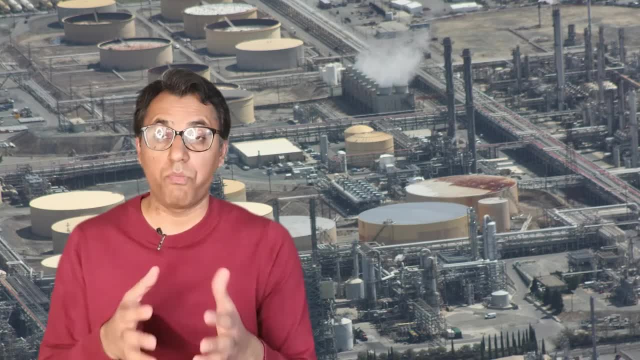 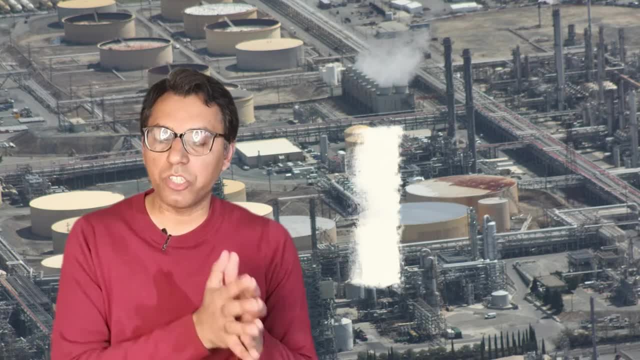 It also provides a more accurate cost and schedule to complete the project before its commissioning starts. It also provides a more accurate cost and schedule to complete the project before its commissioning starts. One of the examples of deliverables of detailed engineering and designs are like including: